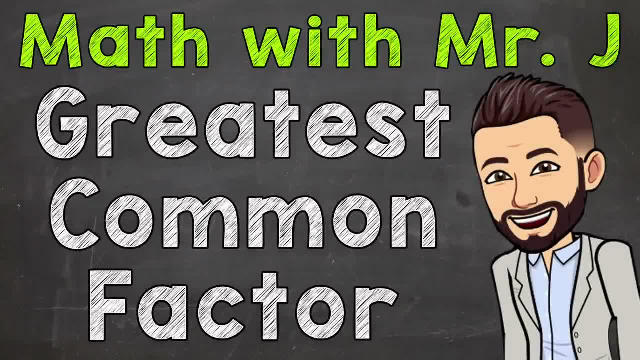 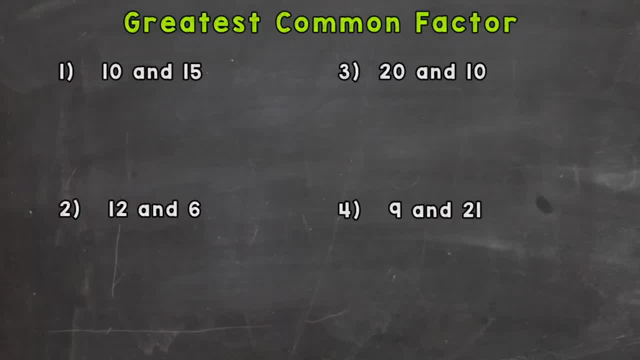 Welcome to Math with Mr J. In this video we're going to discuss how to find the greatest common factor between two numbers- And, as you can see, there are four problems here- and sets of numbers that we're going to find the greatest common factor. So, for example, number one, we have 10. 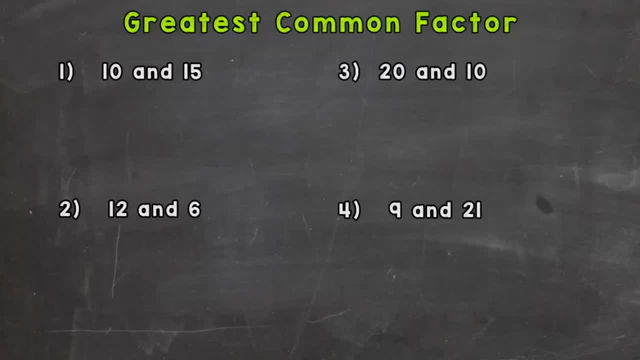 and 15.. So let's jump right into that one and see how we find the greatest common factor. Well before we find the greatest common factor, we need to know what factor means. And a factor are. factors are all the numbers that can multiply together to give you that number. So let's make 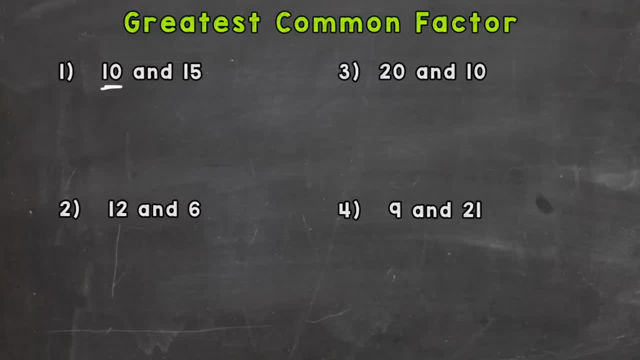 sense of this. So we have 10 here. We're going to list all the factors of 10. And, like I said, it's all the numbers that can multiply together to give you 10.. So for every number, when you're listing the factors, you can start with two things: one and that number. 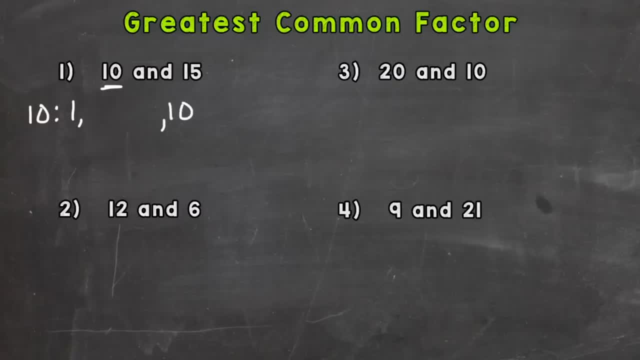 itself, And I'm going to put some space in between for the other factors. These are a factor pair here because I can do: one times 10 equals 10 or 10 times one. That's a multiplication fact that gives me 10.. So those are factors. Can you think of any other pairs that will equal 10?? 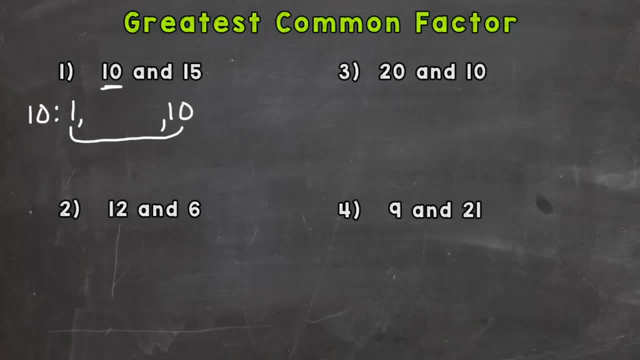 Hopefully you're thinking two and five right, Two times five is 10 or five times two is 10.. So I fill in my space here with the two and the five, And 10 has four factors: one, two, five and 10.. Two and five are a pair as well If you want to connect them. if that helps you out. 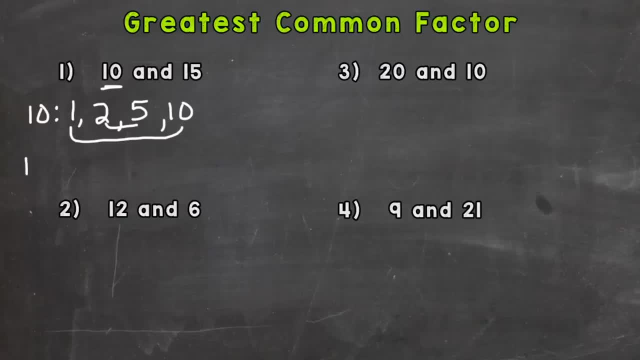 that works, So let's do 15.. So we need to think of the factors Of 15.. So we always start with one and the number itself and leave some space in between for your other factors. Now, once you get better at this, you will get very good at the spacing When you're. 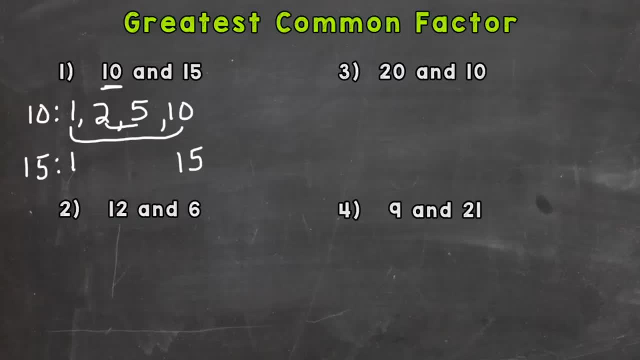 first starting out. you may have trouble spacing out in between there where you can put your factors. That's fine. As long as you have all your factors listed, don't worry so much about the numbers. Sometimes if the number is prime, you'll only have a one and that number itself. That's. 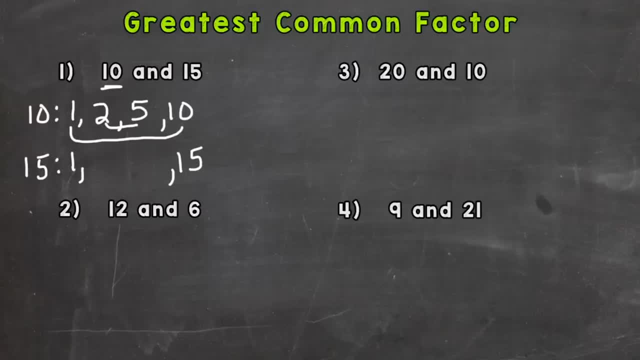 exactly what prime means, But composite numbers means you have more than just one and the number itself. And 15 is composite. So can we think of any other factors for 15?? Hopefully we are thinking three and five right? Three times five is 15.. So three and five are a pair. 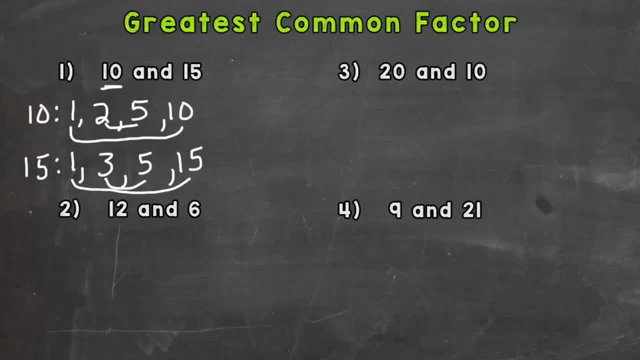 One and 15 are a pair And there aren't any more, So we're done. So now we need to find the greatest common factor, So the greatest one that they have in common. So I see that they have one in common and they also have five in common. So what's the greatest? Well, five, So we can put GCF. 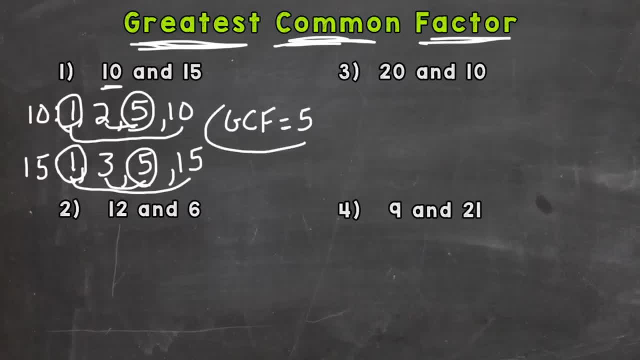 greatest common factor equals five. All right, let's try number two here. So we have 12 and six. Let's start with our factors of 12.. So we start with one and 12.. Well, 12's even So. I know two is going to be a factor And you can. 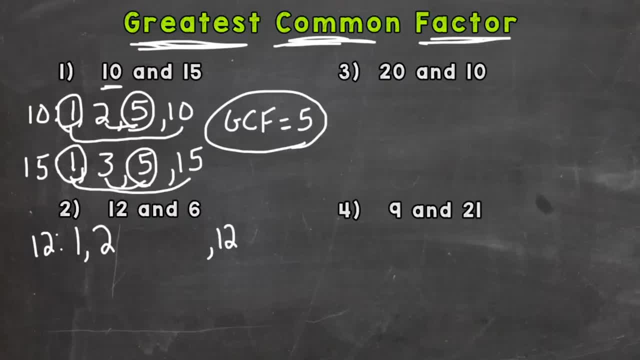 think: well, what's two's partner? Well, six, two times six gives me 12.. So put my six here, And there's one more pair or two more factors for 12.. and it's 3 and 4, and that's it for 12. now let's write our factors for 6, so we 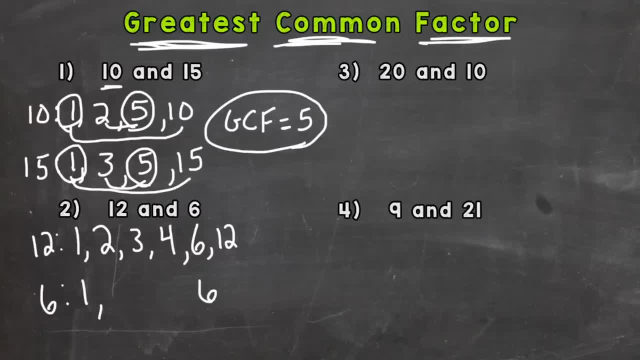 always start with 1 and the number itself, 6, is. even so, I know 2 is automatically going to be a factor and 2's partner or other factor for 6 is 3 here. so there's your list of factors for 6. so I see they have 1 in common and 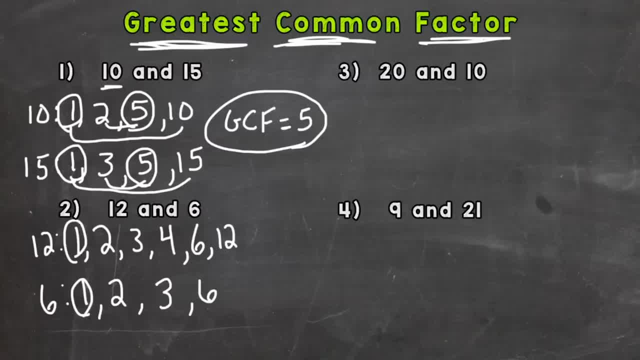 sometimes that will be your answer for greatest common factor, not for number 2 here. well, speaking of 2, they have 2 in common, 3 in common and they also have 6 in common. so they have a lot of common factors, but we want the greatest, so the. 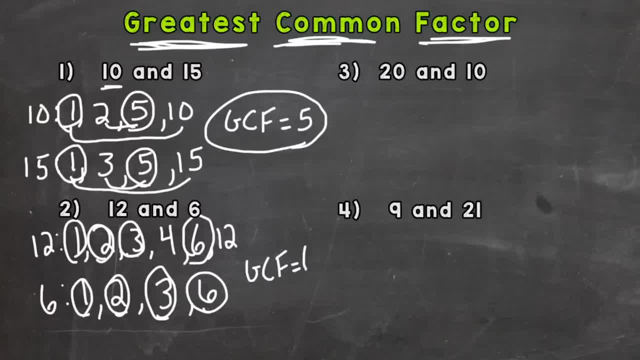 GCF for 12 and 6 is going to be 6.. all right, number 3 and 4 here. if you feel comfortable enough to try a couple on your own, feel free to press pause, finish 3 and 4 and then when you're. 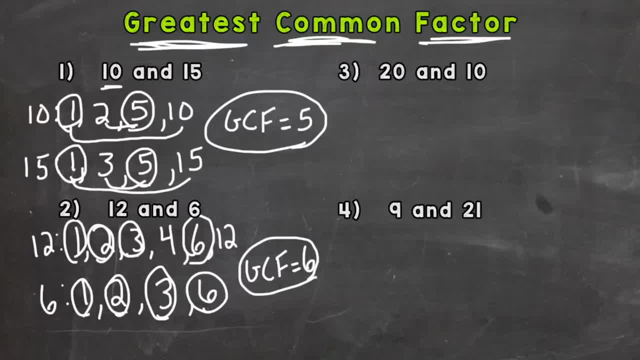 ready, press play and check your work with mine. if you want to do 3 and 4 with me, that's fine as well. so let's do 20 and 10. so we'll start with 1 and 20, and I know that 20 is even so. 2 is going to be a factor and his partners 10, any. 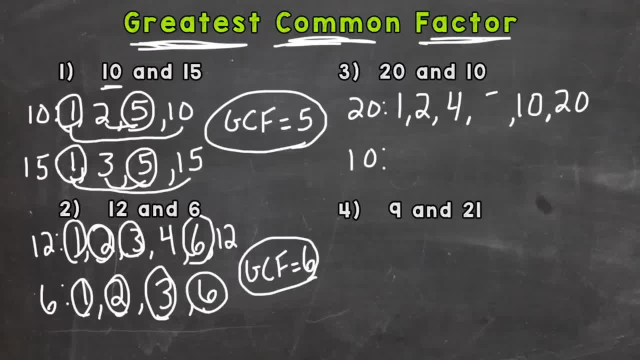 others. well, 4 & 5, and that's actually it for 20. so let's do ten, one and ten, and when you get into greatest common factors, one thing you should look for is if you already have a list of Xiид and Symphony on your livings, then you should put them in a list if you're comfortable with the most usual discrimination. 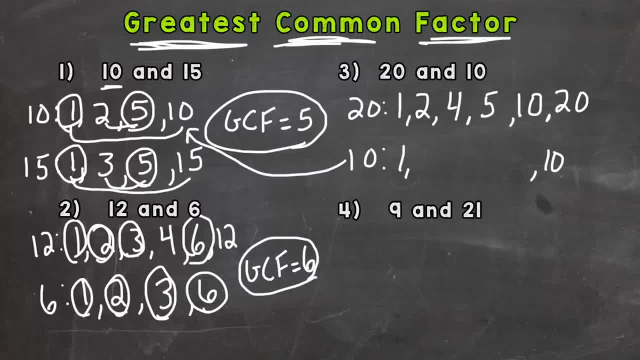 something. Use it, And we know that 10 is 1,, 2,, 5, and 10.. Notice, my spacing wasn't great on that one. I have a lot of extra space here. That's fine. I have all my factors listed and that's. 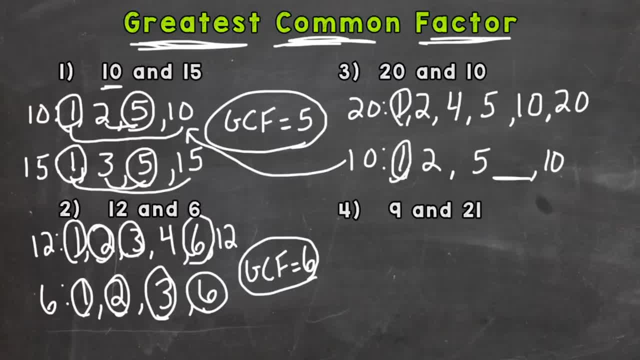 the most important part. So I see that 1,, 2,, they have 5 in common and then they have 10 in common, So the GCF is 10 for 20 and 10.. All right. lastly, number 4. We have two odd numbers here, 9 and 21.. 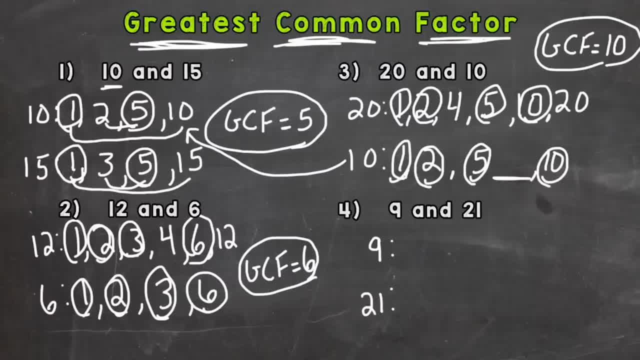 So let's write our factors. So for 9, we'll start with 1 and 9.. And then is there anything else that we can multiply to get 9?? Well, 3 times 3.. So 3 is a factor. You only need to.